a year to maintain and they're often on valuable real estate. Most cities don't even know what to use them for after the games. Those facilities fall into decay if they're not kept up and that hurts property value. It could also be a lot of environmental disruption. The Winter Olympics they'd be having in. 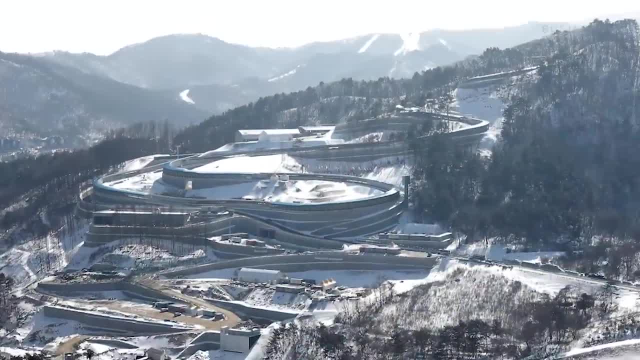 Pyeongchang. they destroyed a whole mountainside, Trees and trees. It could also be a lot of environmental disruption- The Winter Olympics they'd be having in Pyeongchang. they destroyed a whole mountainside, Trees and trees. It could also be a lot of environmental disruption The Winter Olympics they'd be having in Pyeongchang. they destroyed a whole mountainside. 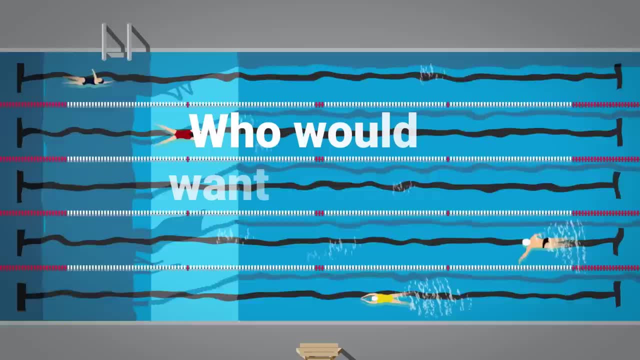 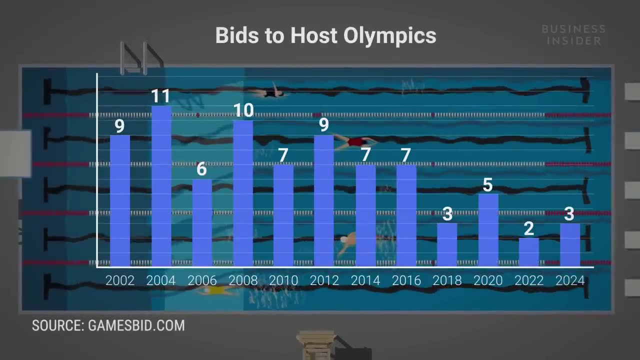 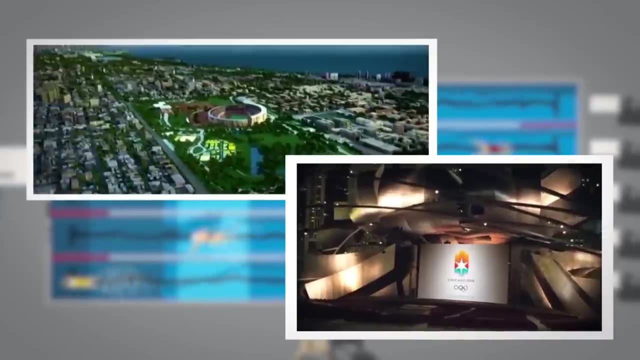 Trees and trees. So who would want to host the Olympics in the first place? Not many. After each financial failure, fewer cities bid to host the following decade's games. After all, it takes 10 years of planning just to be in the running. to host, Chicago spent an estimated $100 million on. 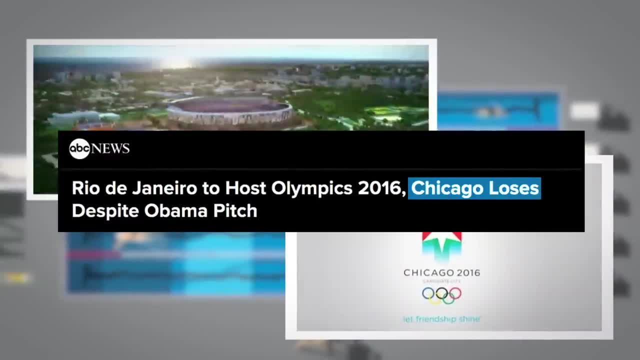 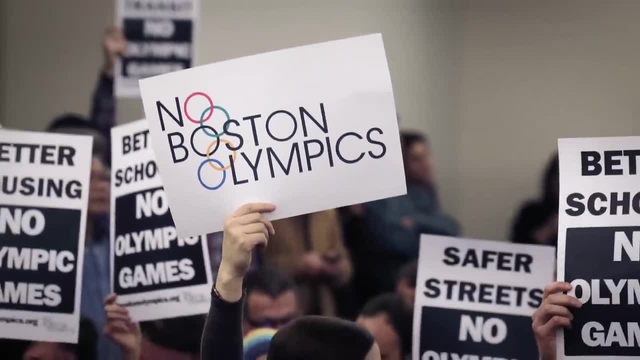 the campaign to host in 2016, and they lost. Boston famously pulled its bid for the 2024 Summer Games after Citizen Group noted that no Boston Olympics convinced the city. otherwise, 12 cities bid for the 2004 Games, five for 2020,. 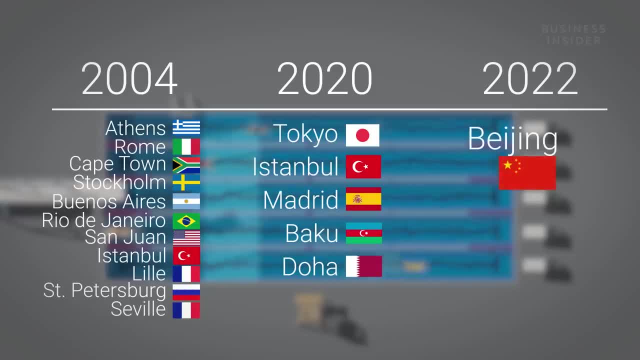 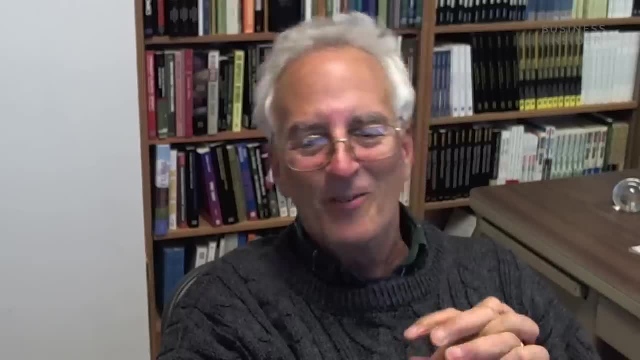 and just two tried for the 2022 Winter Games: China and Kazakhstan. So is that it RIP Olympic Games? Oh no, it won't end. Thomas Bach, the president of the IOC, for all the criticisms that I have of him. 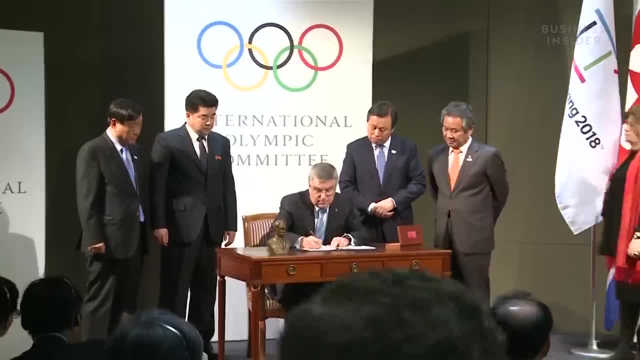 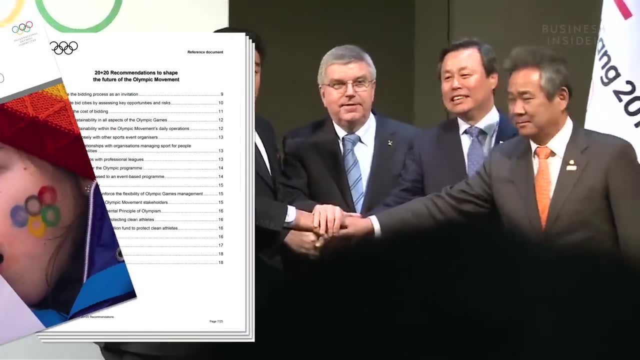 he's a smart guy and he knows when he's up against the wall, and they've been up against the wall. In 2014,, IOC President Thomas Bach suggested a list of 40 actions the IOC could take to shape the future of the Olympic movement. 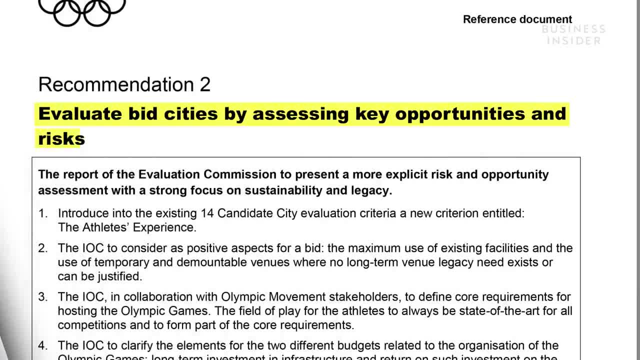 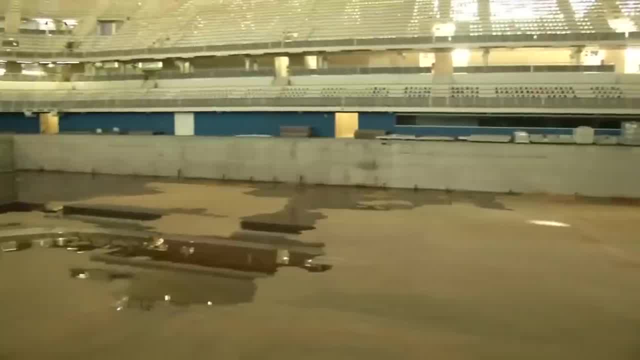 Among them: evaluate bid cities by assessing key opportunities and risks, reduce the cost of bidding and include sustainability in all aspects of the Olympic Games. It sounds good on paper, but time will tell. if these actions take root, We're gonna become more sustainable. 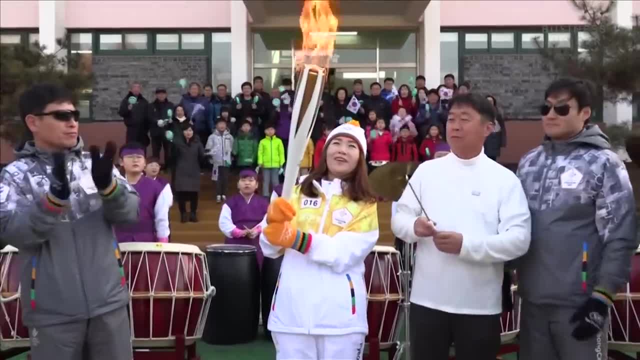 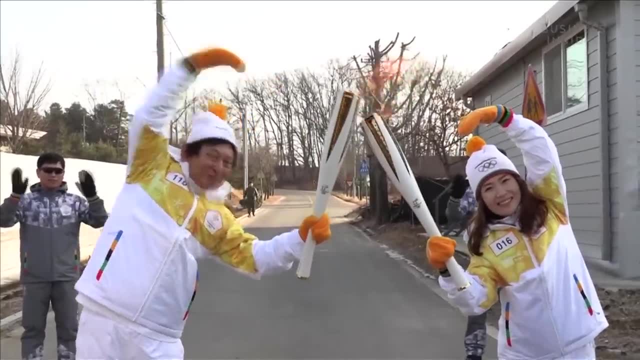 we're gonna become more affordable, we're gonna become more flexible And by doing that, by tweaking the model a little bit, making pronouncements, they reengage cities to participate, And what's generally happened is the model has been slightly reformed. 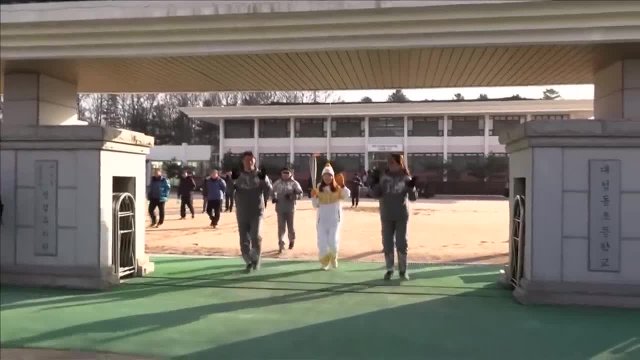 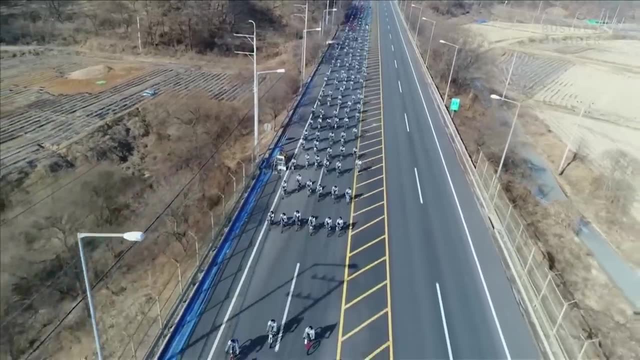 It's a little bit more sensible now than it was before Agenda 2020.. Zymbolis supports a different idea: to keep the Olympics alive, Get rid of the bidding system and pick a permanent host somewhere that has the built-in facilities, infrastructure and venues.